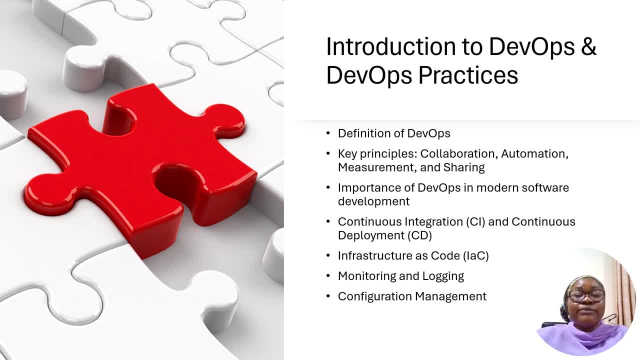 This allows us to provision and manage infrastructure using version-controlled code, Bringing consistency and scalability to our deployments. Furthermore, monitoring and logging are essential in DevOps. We must build systems that can be monitored in real-time, providing insights into performance and user behavior. 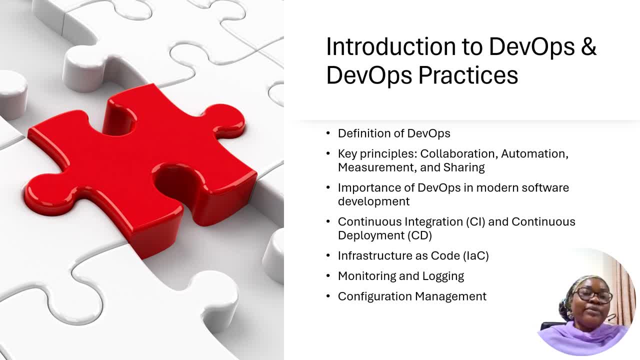 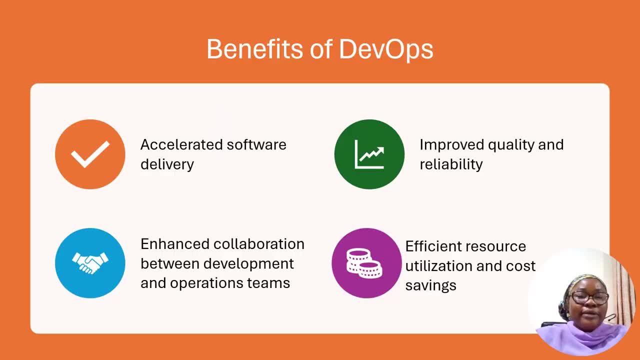 The data-driven approach enables us to make informed decisions and continuously optimize our applications. Now let's talk about the benefits. DevOps accelerates software delivery, shortening the time from cold commits to production. Now let's talk about the benefits. DevOps accelerates software delivery, shortening the time from cold commits to production. 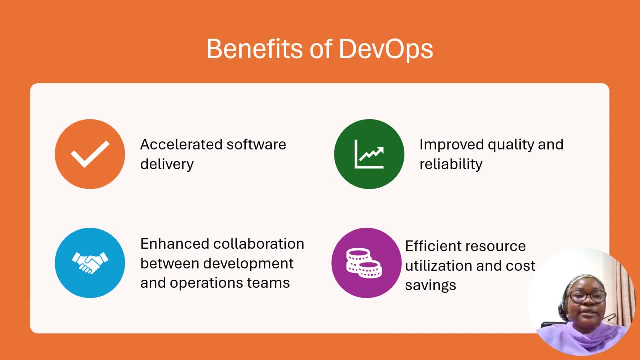 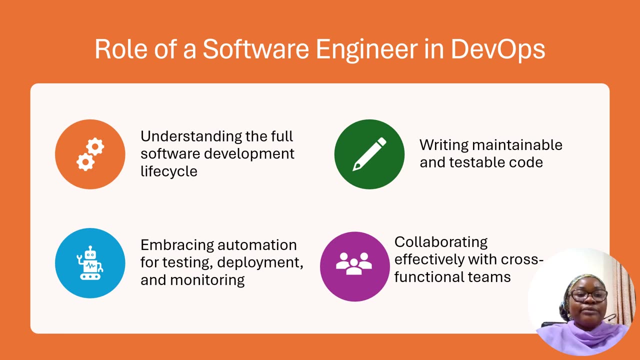 It improves the quality of our software through automated testing and feedback loops. Collaboration between teams is also enhanced, breaking down barriers and fostering a culture of shared responsibility As software engineers. in the DevOps world, we need to be versatile. We must understand the entire software development lifecycle. 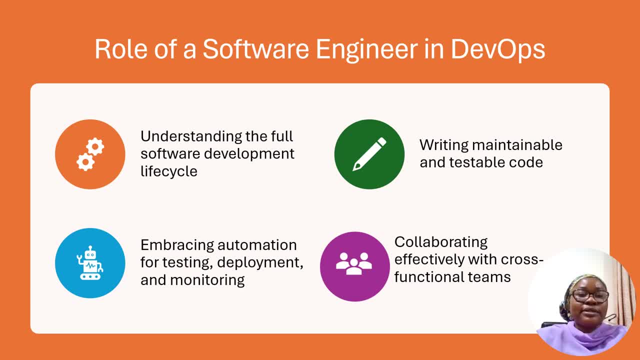 From design to deployment. we write code that is robust, scalable and secure. We embrace automation using tools to streamline counseling, marketing and戰異 Chinese Hil運. We embrace automation using tools to streamline responsible management tasks. We embrace automation using tools to streamlinerating infrastructure and diplo sting. 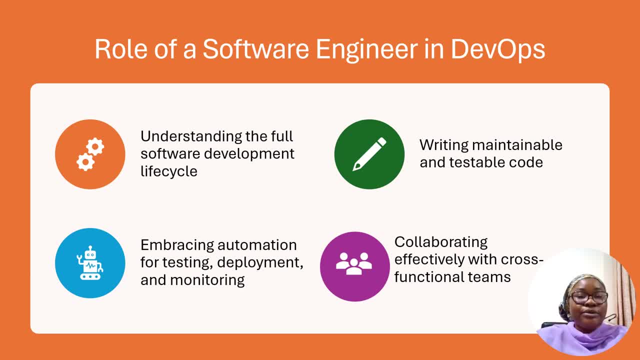 We will overcome difficulties with Godlair for 2021.. We are build cookies, We promote capabilities using complexоров, county characteristics and cars, plan repetitive tasks and focus on innovation. So, in conclusion, DevOps is not just a methodology. 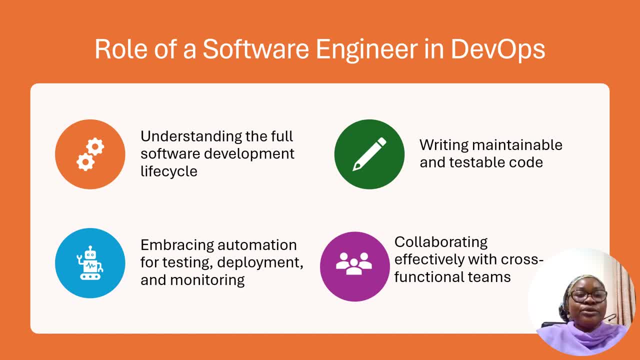 it's a mindset. It empowers us to deliver value to our users faster and with higher quality. So, as software engineers, let's embrace DevOps principles, collaborate across teams and leverage automation to build the future of software together. Thank you for your attention. 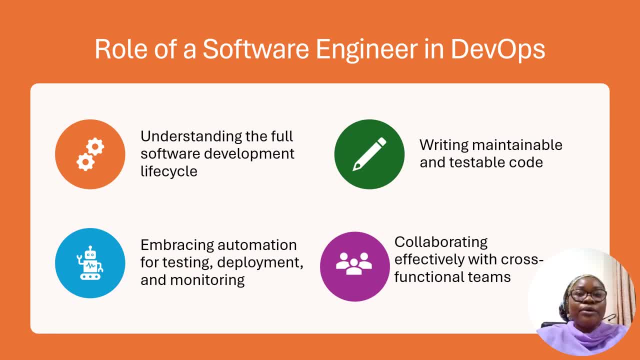 Let's continue this journey of learning and innovation in the world of DevOps.